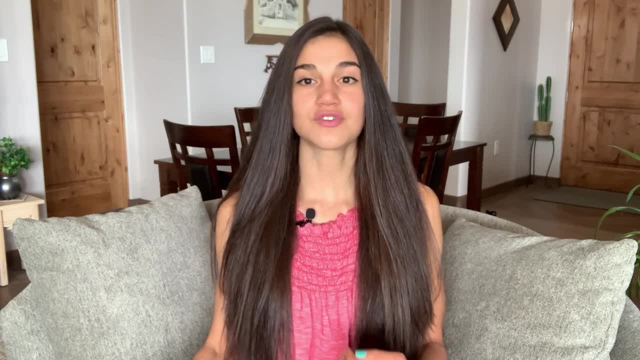 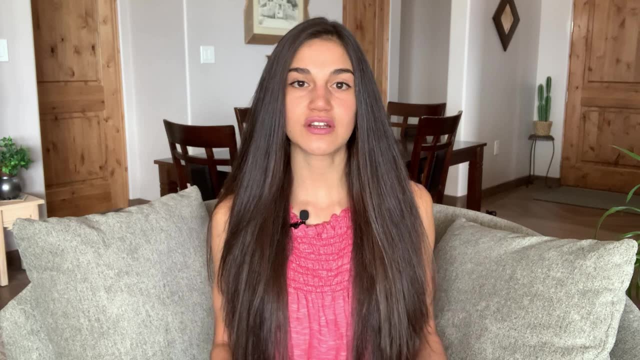 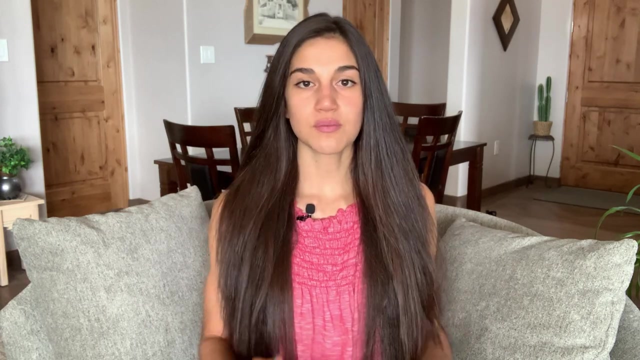 they could determine your salary as well as what kind of degree you'll be getting. So, with that being said, I'm going to first explain what computer engineering is. So computer engineering is basically the understanding of the hardware and software integration As a computer engineering. 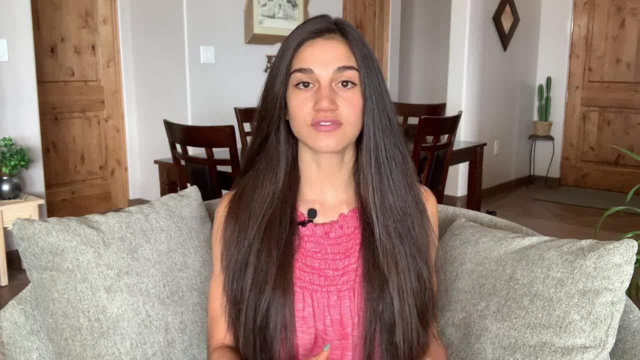 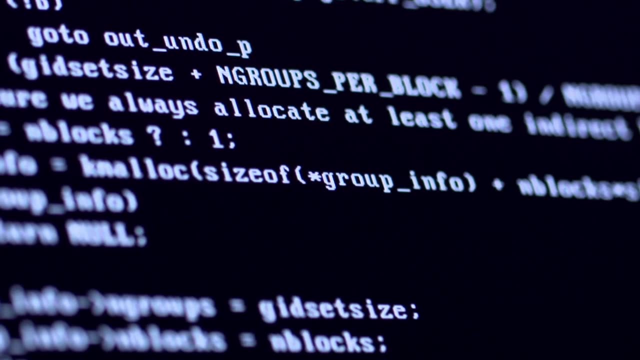 student, you understand how the software applications are developed, the back end of the program and how the software applications are developed, So the background of the program and how basically an application on a particular computer or a laptop or on a hardware is created, As well as understand the hardware that the application is running on. So, for example, 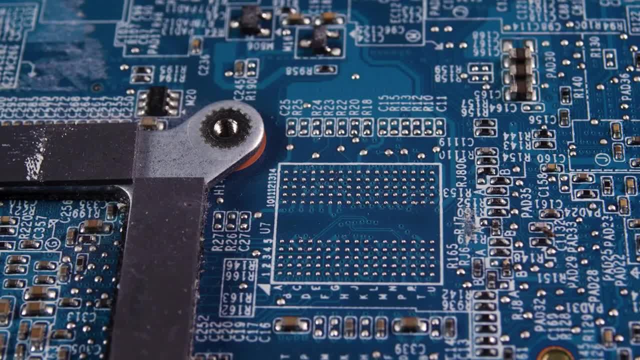 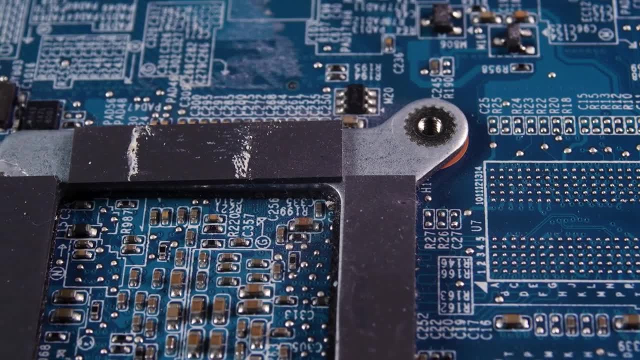 the architecture of the computer. You understand what you know. memory is what, the ram is the way in which the operating system stores data and where it stores it, and how it divides it up, and what methods it uses to store this data, As well as how. 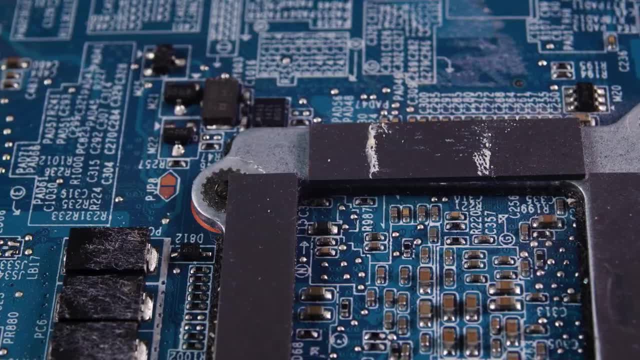 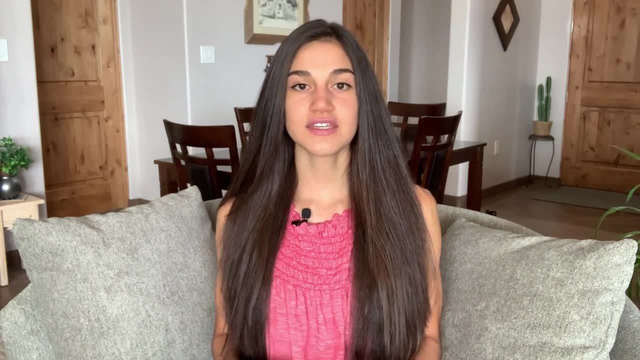 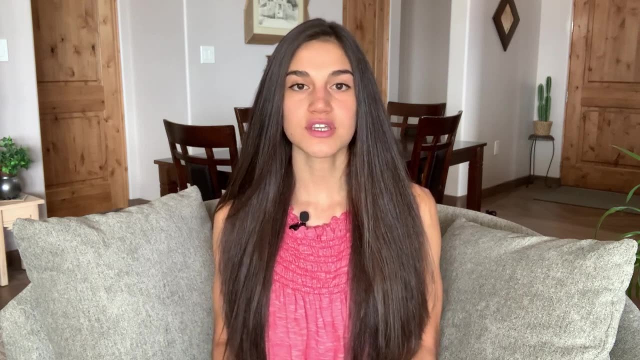 it supports these applications so that they can run on this particular computer. So that's all computer engineering. It's the understanding of both the software and the hardware side of things. IT, on the other hand, is where you are using and maintaining the software that has been developed. For example, IT could be those who are fixing a particular 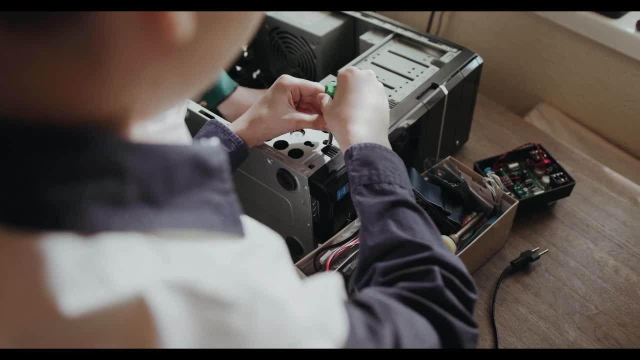 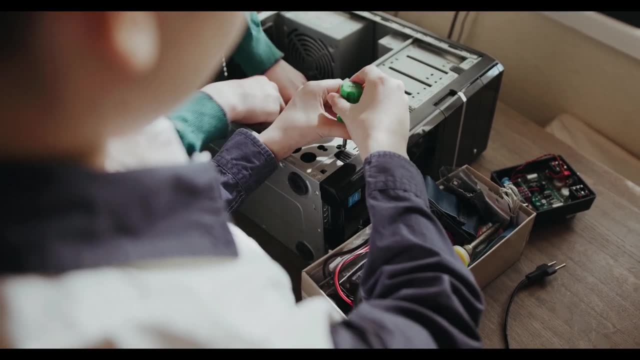 hardware, rewiring a particular microcontroller, repairing a computer by either restoring the OS system or getting new parts, or reassembling the computer, whatever it may be. They're the ones who make sure that the computer is back up and running again. So they maintain that computer. 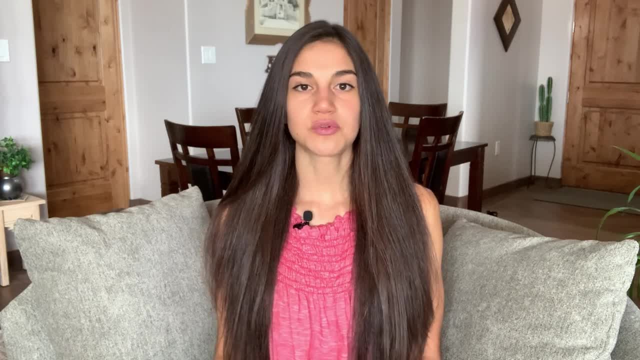 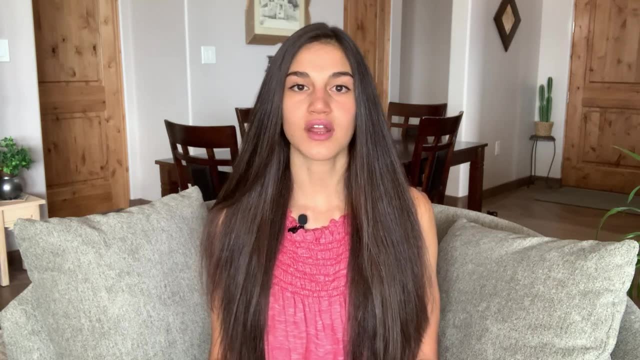 With the software. they maintain the programs. For example, the program were to break and someone needed help, then they would look and see what do the instructions say on how to use this particular software in this program, And they'll either rerun the application, uninstall it, reinstall it. 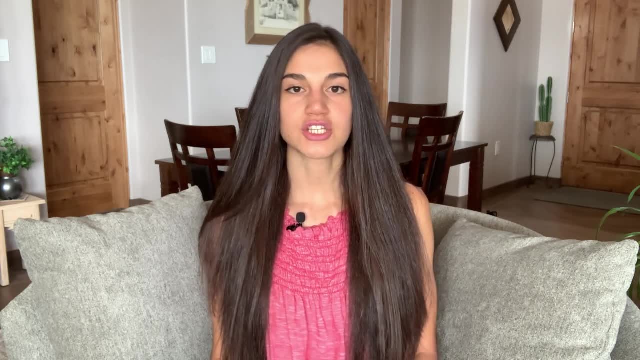 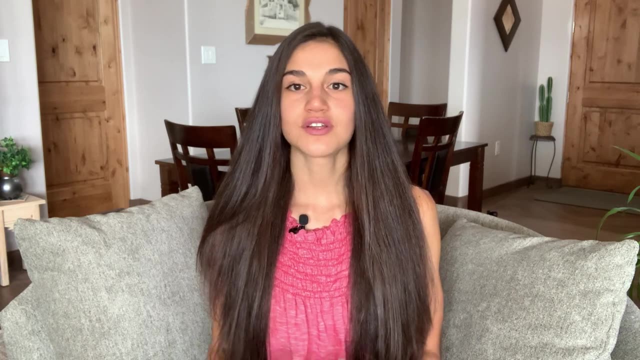 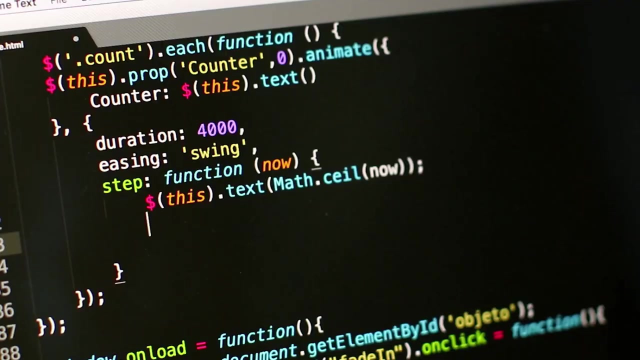 run different commands to reconfigure the application or reset the settings within the application, whatever they need to do to get it back up and running again. That's where the distinction lies. That is a huge distinction because computer engineers can become computer scientists. They know and understand how software applications are programmed and how they're built. 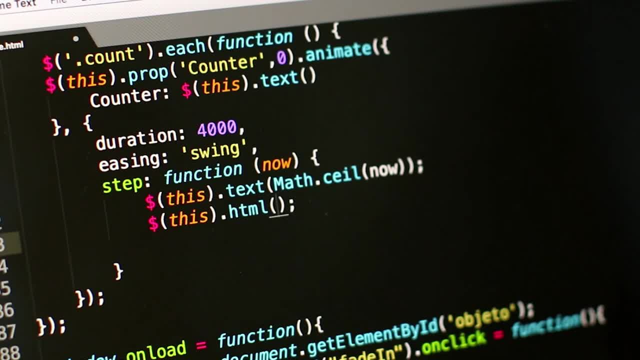 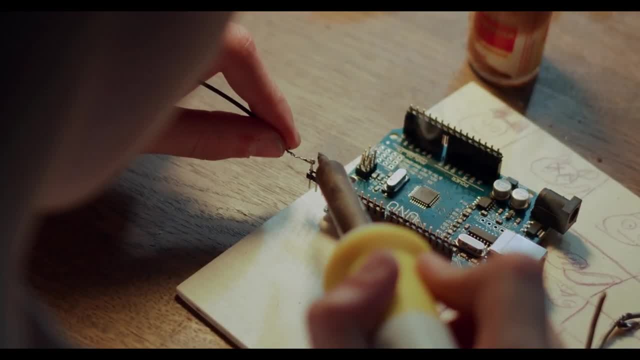 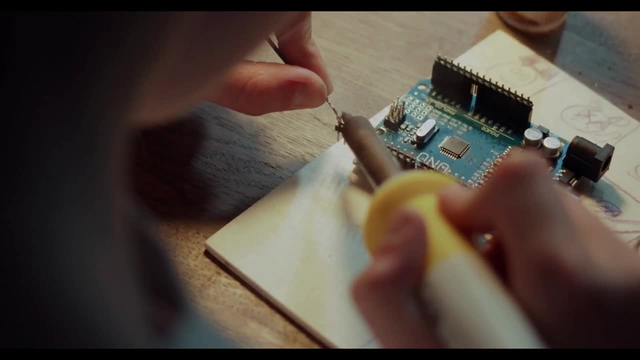 So they could become a computer programmer and build applications themselves if they want. And same with the hardware. They understand how the mechanics work within a computer. They understand the CPU, the microprocessors, the circuits within the microprocessors and how that's all run. So because of that they could create. 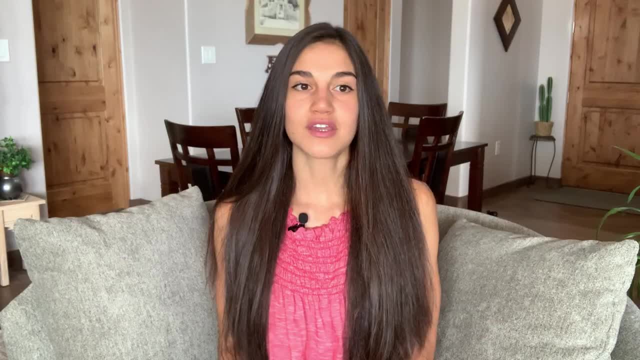 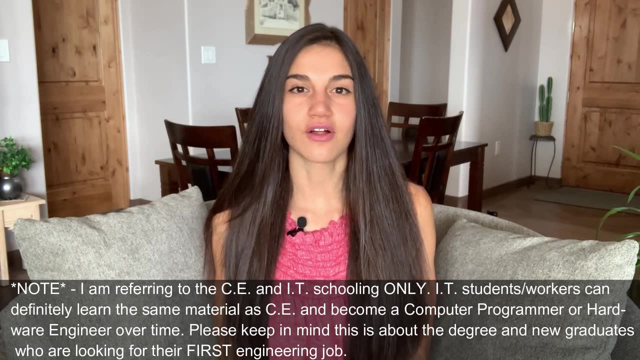 their own microcontroller and thus their own computer if they want, because they have that knowledge and that background, Whereas IT they would not be able to do that because they don't have that knowledge or background. They wouldn't be able to become a computer scientist and program. 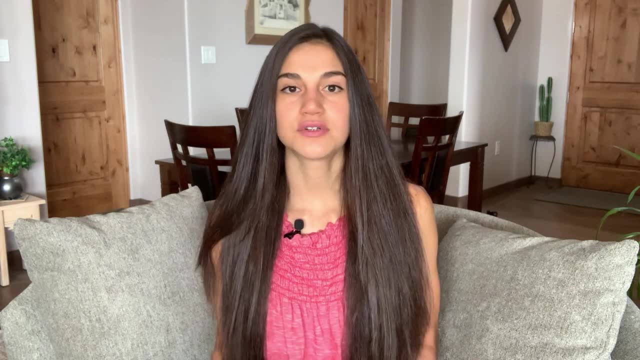 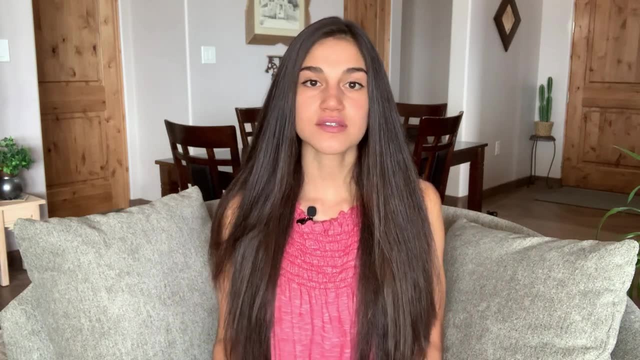 a software application or become a hardware engineer and create a microcontroller or a computer by themselves. And the other thing is that computer engineers, in order to understand all of this, because it's a lot of information, they would have to get a bachelor's. degree in computer engineering. So you'd have to go for four years to become a computer engineer, Whereas with IT you'll only need an associate's degree most of the time. So you'll only need to go to school for two years, because there's not as much information you need to know. But because of that computer engineers do get paid more than IT. Now, that's not to say that IT employees can't get paid more than the average computer engineer. I'm sure there's plenty of IT workers who get paid above you know $150,000 or something, but they've been senior IT employees and they've been working there for much, much longer, Whereas with computer engineers there's a lot more computer engineering students who just got out of college making at least $100,000 a year And then from there it just goes up. So it really is a give and take with. 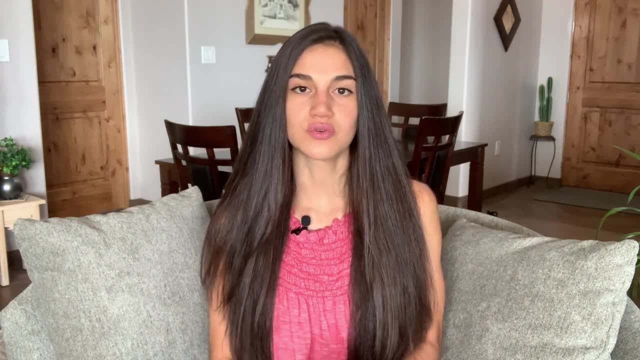 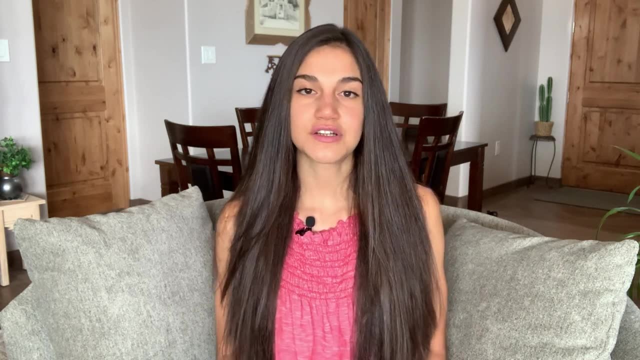 computer engineering versus IT. in terms of the salary and the school, It really depends on you and your personality and the person. It's very individualized. I got an engineering degree, so I, of course, am on the side of computer engineering. 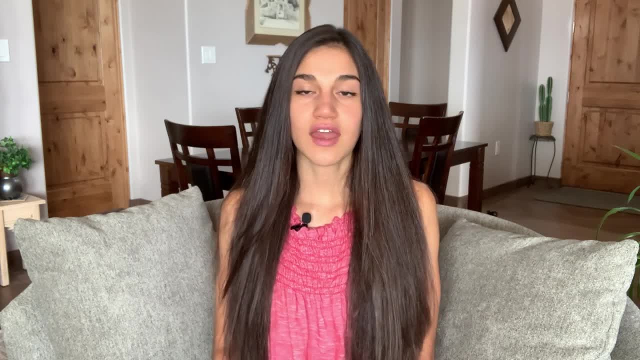 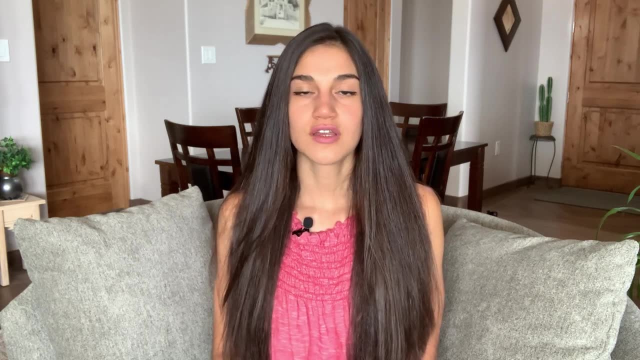 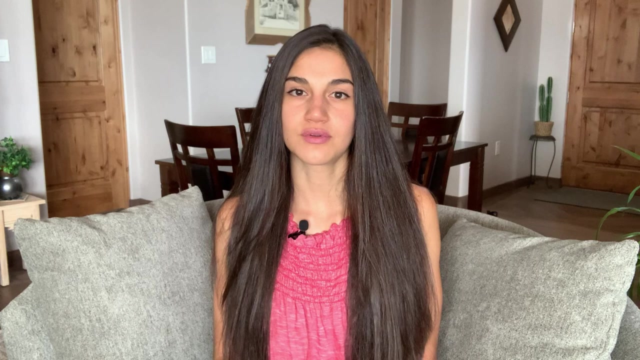 If you would prefer doing IT, then that's great. I think both of them have high prospects. It's just that it depends on what you would like to do more. Would you rather create the programs and create the hardware, or use and maintain the hardware and software? So that's up to you. 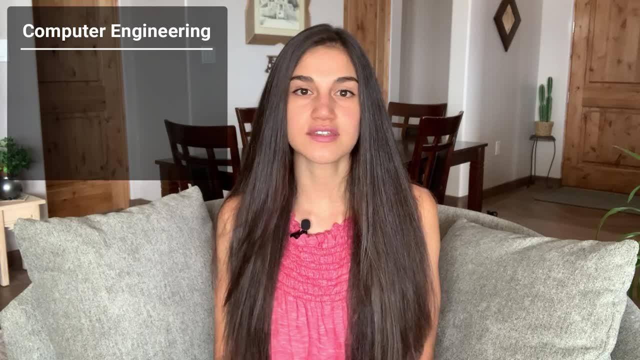 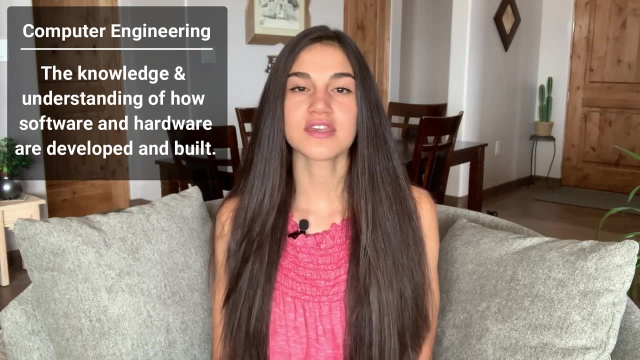 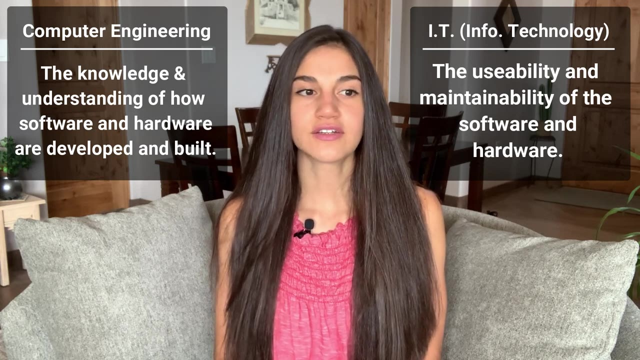 But those are the two distinctions. So, in summary, computer engineering is basically the knowledge and understanding of how the software programs are built and how the hardware is built, Whereas IT is the usability and maintainability of the software and hardware. So that's all I have. I hope this clears it up a bit, And if it didn't, or if there's something, 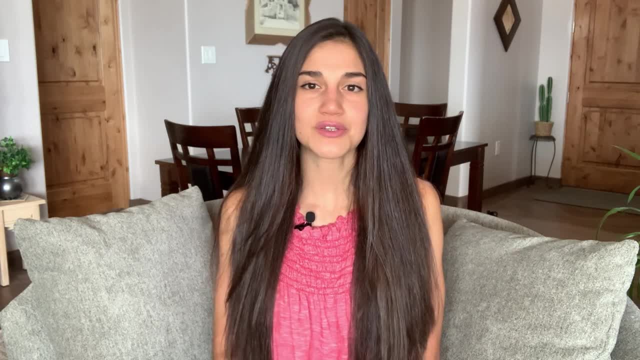 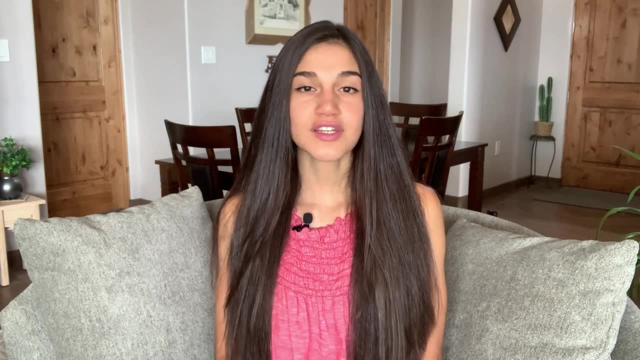 that I missed, please let me know in the comment section down below, and I could definitely make a part two and go in more detail about these two subjects. But other than that, I hope you guys found this helpful and useful And if you would like to see more videos in the future,